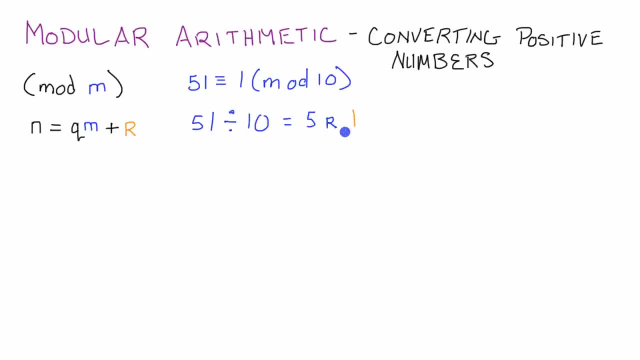 And that gives us the result 5 with a remainder of 1.. 10 goes into 51 5 times, and then we have 1 left over. When we're dealing with positive numbers. that's really all you need to do to convert that integer into a number within the mod. 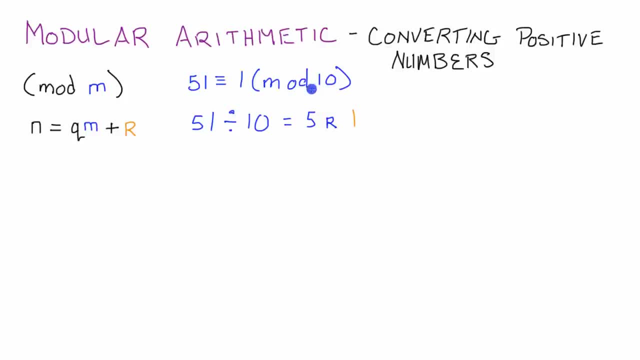 So 51 maps to 1 when we're dealing with mod 10.. So this is pretty simple when we're dealing with positive numbers, but when we're dealing with negative numbers it's a little more tricky. So I want to go ahead and use this formula over here to get a more clear. 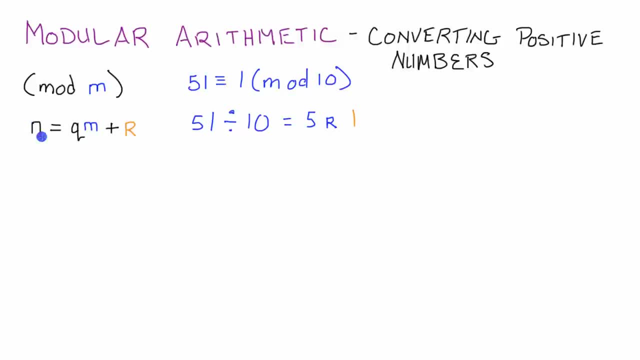 representation of what's happening. So n right here is going to represent the number that we're originally starting with. In our case it's 51.. 51 is the number we want to convert so that we can use it in mod 10.. 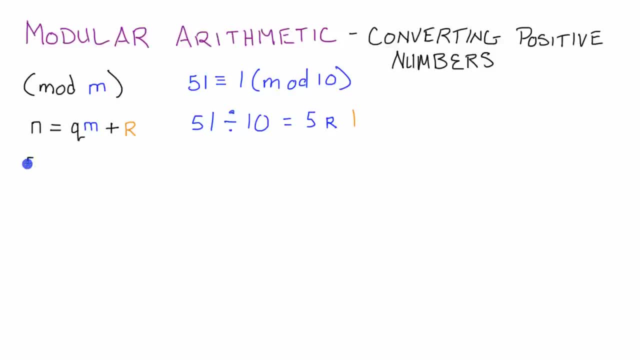 So in this case n is 51.. So we'll just go ahead and write that below the n And that's equal to some number. q and q can be whatever we need it to be for this to be an equivalent statement here. 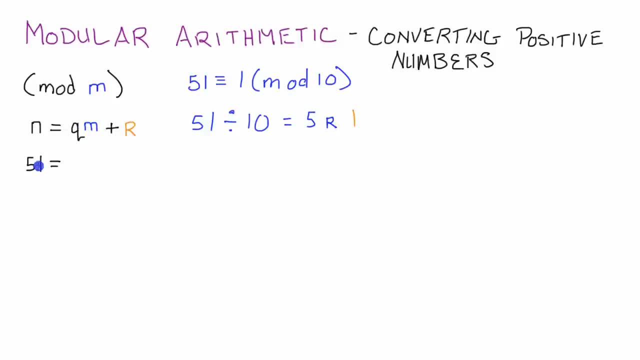 In our case q, is this 5 right here? So 51 is equal to 5.. And then qm means q times m or 5 times, in our case m, here Mod, m, mod, 10.. 10 and m are the same thing here. 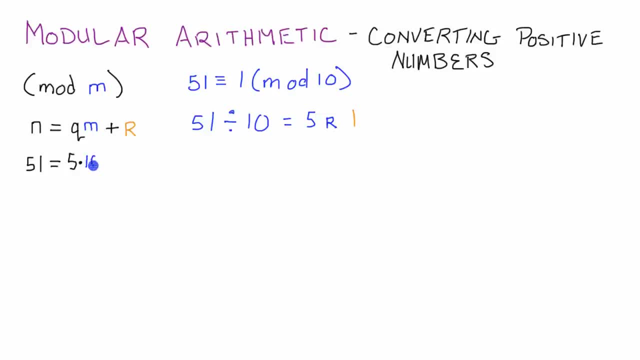 So in our case the m or the mod is 10.. So 51 is equal to 5 times 10, or simply 50, plus a remainder of 1.. 51 is equal to 5 times 10, or 50 plus 1.. 50 plus 1 is 51.. 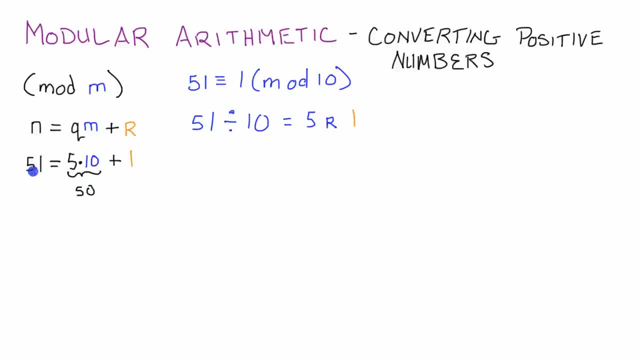 So when we're dealing with positive numbers, we don't really need We don't really need to write it out like this, But I find that writing it out with this equation: n is equal to qm plus r. it's really helpful when we start converting negative numbers to fit within our mod. 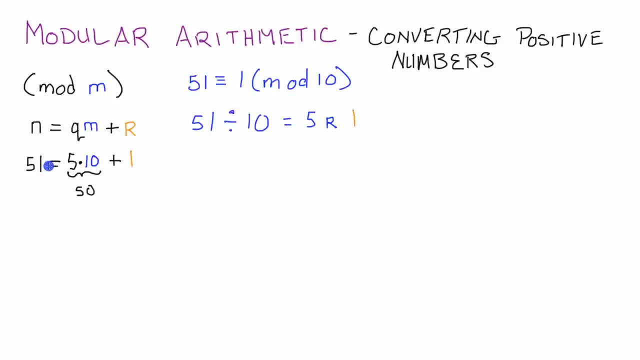 So let's just do a couple more examples of this with some positive numbers, And then in the next video I'll go ahead and use this same formula here to show how to convert negative numbers so that they fit within our mod as well. So let's look at 27.. 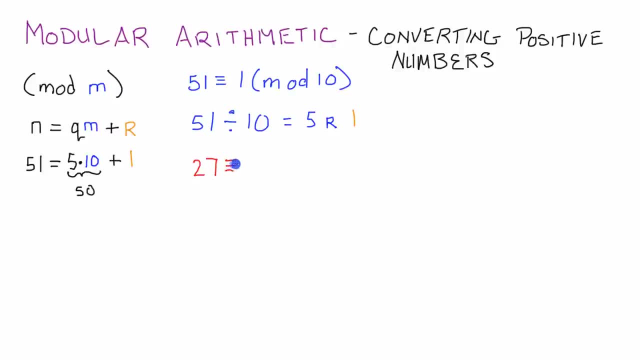 And we want to know what number 27 is congruent to when we're dealing with mod 6.. We can simply take the 27 here and divide it by the mod, which is what we did here up above in this example. So we're going to do the same thing. 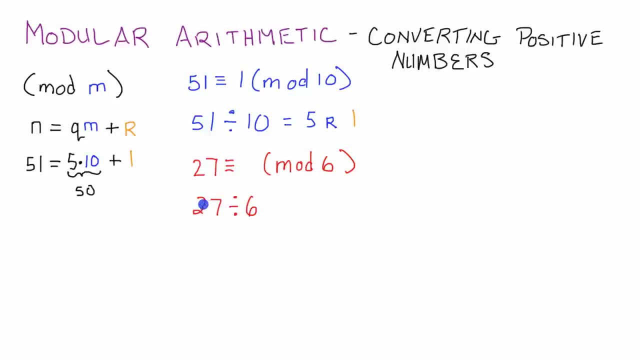 27 divided by 6.. 6 goes into 27, four times, with a remainder of 3.. So if we write that in this n is equal to qm plus r formula, it's going to look like this: n is the number we started with, which is 27.. 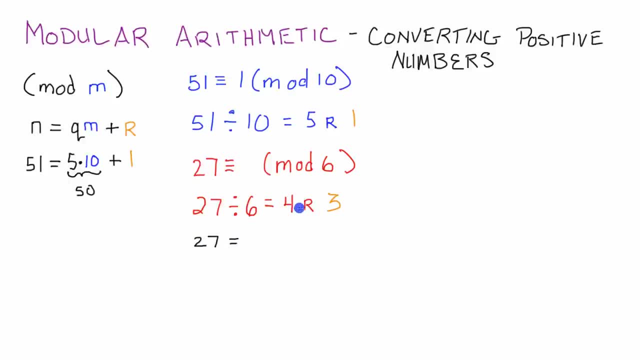 So there's our n, That's equal to q. In this case, the q would be the 4. here times m, m is our mod. We're dealing with mod 6 plus r, which stands for remainder, And in this case our remainder is 3.. 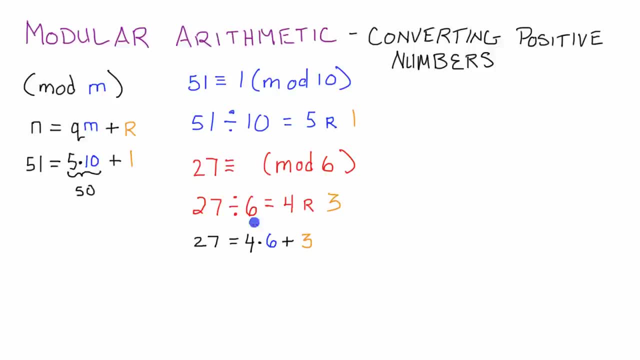 And if we can make this a true statement, then that just means that our remainder is what we convert our original number to when we're dealing with that particular mod. So in our case, 27 converts to 3 when we're dealing with mod 6.. 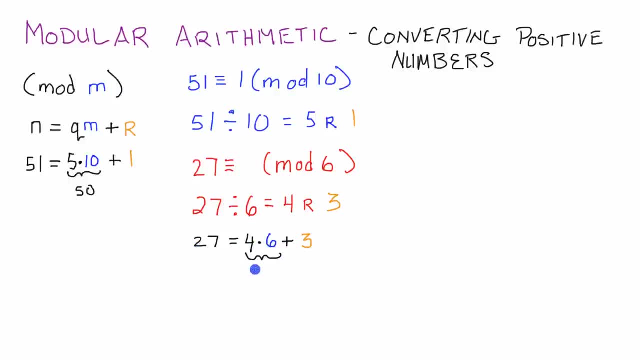 So 27 is equal to 4 times 6,, which is 24 plus 3.. 24 plus 3 is 27.. So this works out. So 27 is congruent to 3 when we're dealing with mod 6.. 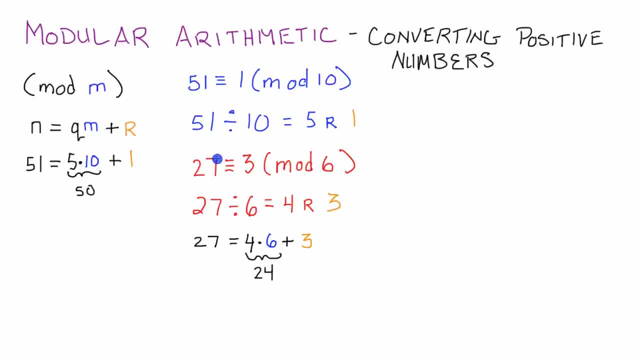 So let's do one more example where the number we're trying to convert is less than the mod, but still positive. So let's say that we're looking at 3, and we're trying to convert that to some number in mod 4.. 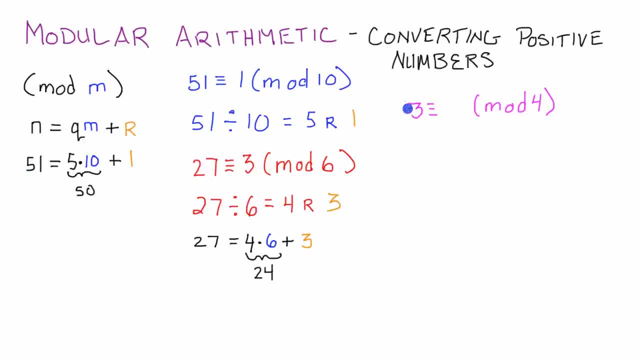 So, using the same approach here, our n is the number we want to convert, So that would be 3.. We take 3. And we divide it by our mod. In this case it's 4.. So 3 divided by 4 is equal to 0, with a remainder of 3.. 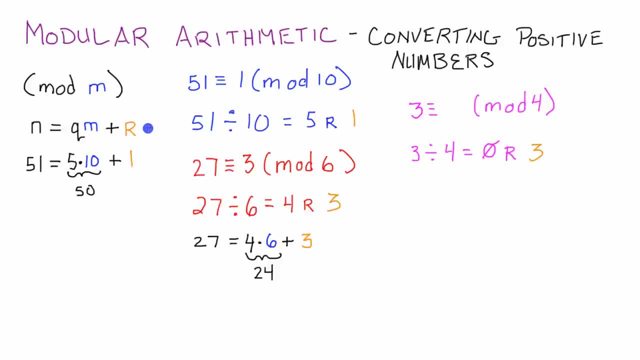 So rewriting it in this n equals qm plus r form. our n is the original number, So that's 3.. And that's equal to this number right here, which is 0 times our mod. In this case, our mod is 4 plus the remainder 3.. 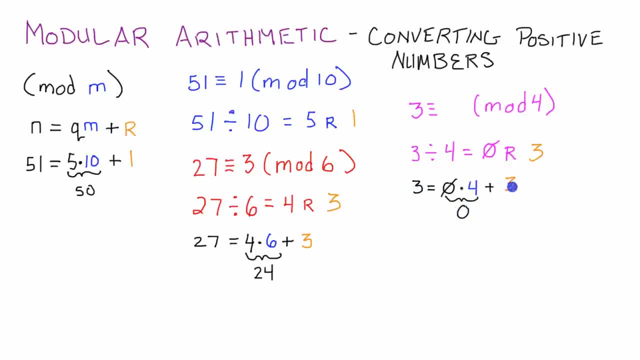 So essentially 3 is equal to 0 plus 3.. 0 plus 3 is 3.. So in this case we don't really need to convert 3.. It's already within the mod. So if we couldn't already tell before we started, if we went through the process we would find out that we don't need to convert 3 to keep it within mod 4..